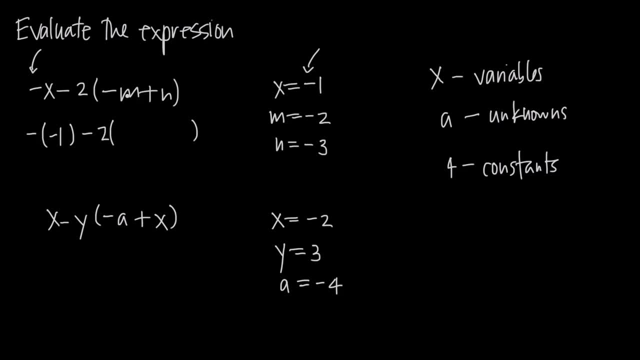 are parentheses around negative m plus n For negative m. again, we need to keep this negative sign and this negative sign. so we'll have a negative, negative 2 when we put parentheses around the m and we plug in this negative 2 value for m And then we want to plug in. 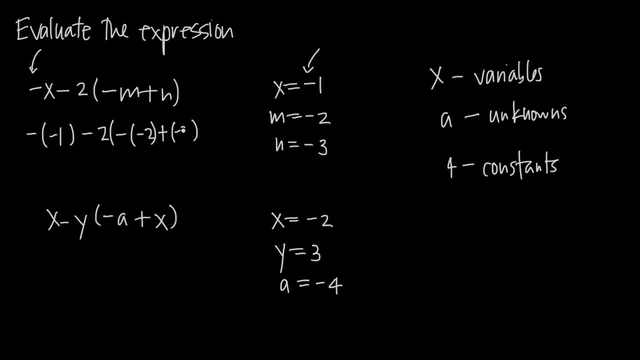 negative 3 for n. so we'll say plus and then in parentheses, negative 3.. And now that we have everything plugged in, it's just a matter of order of operations. we want to go ahead. do the values inside our parentheses first. so we'll do the values inside these parentheses here. 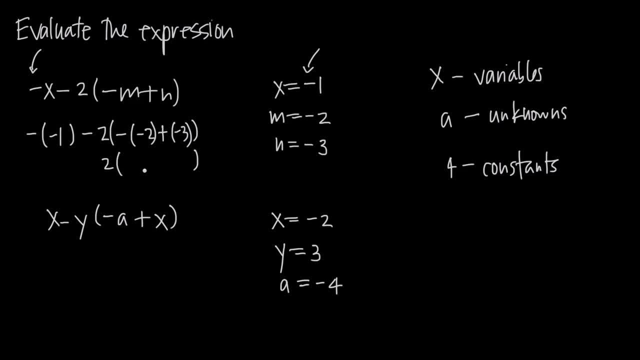 a negative negative 2. that tells us we're taking the opposite of negative 2, which we know is a positive 2. and we know that also because we can cancel every two negative signs to get a positive and then we have a plus negative 3. those are different signs. there's only one negative sign. 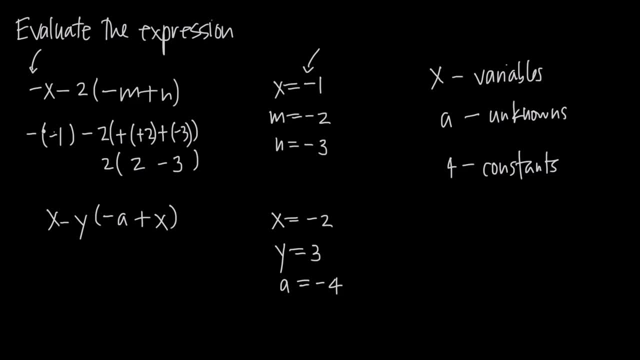 so this turns out to be a negative 3 or just minus 3, and then we have a negative, negative 1 or the opposite of negative 1. we can cancel those two negative signs to get a positive and we have 1 minus. now we're going to simplify the value inside our parentheses, so we'll get 1. 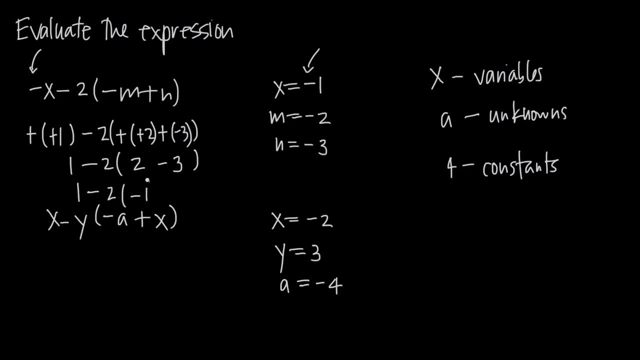 minus 2 times 2 minus 3 is a negative 1, and then, if we take this over here, we'll multiply the 2 by the negative 1. 2 times a negative 1 is a negative 2, so we get 1 minus a negative 2, or. 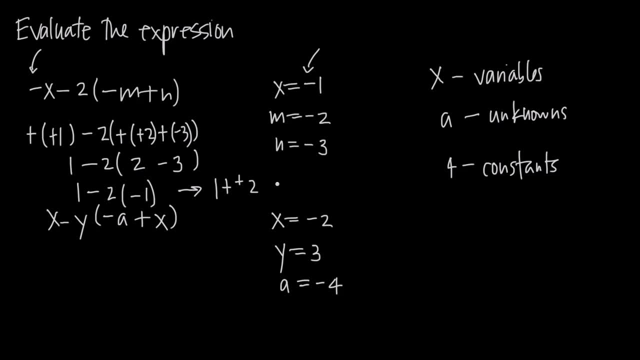 canceling these negative signs, they become positive. 1 plus 2 is going to be equal to a positive 3, and this is the value we get when we evaluate the expression. given these values for the variable x minus y times the quantity negative a plus x, We know that x is negative 2,, y is 3, and 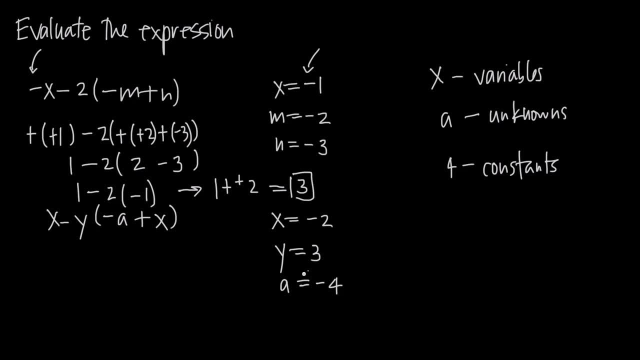 a is negative 4.. So we're just going to be plugging in these values again, So plugging in a negative 2 for x- we have x out in front here, so we'll get a negative 2, and then we have minus y here we know is 3, so we have 3 times the quantity here: negative a plus. 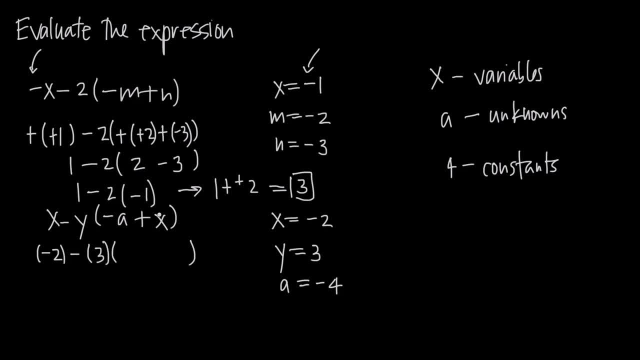 x. We have a is negative 4, but we also have this negative sign, so we'll say a negative negative 4, and then plus x. we know x is negative 2, so we'll say plus negative 2.. We can bring this negative 2 outside of the parentheses, so we'll get negative 2 and then